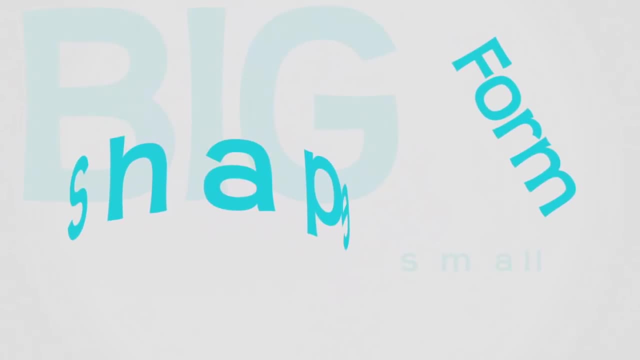 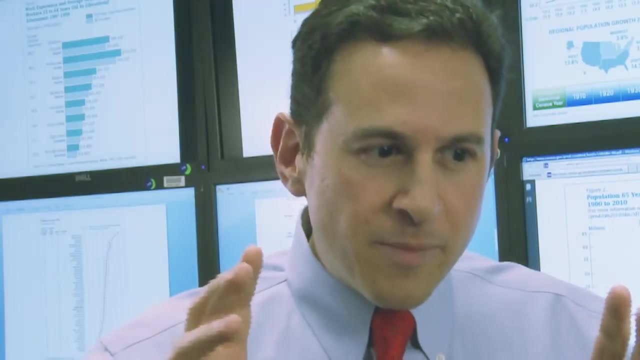 shapes are what their form is. If you can get the form, you can get the function and you can get some understanding. You want to build a microchip. You need a microscope. Now that means that a microscope is really really useful for looking at things that are: 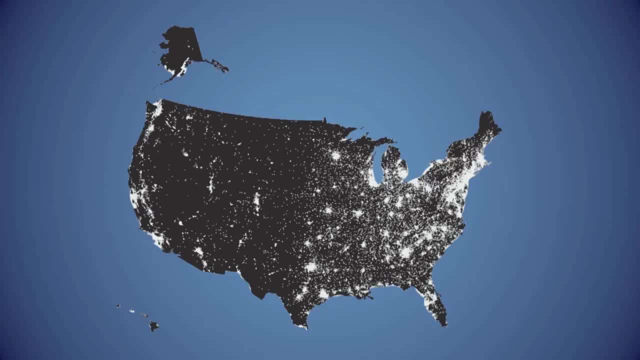 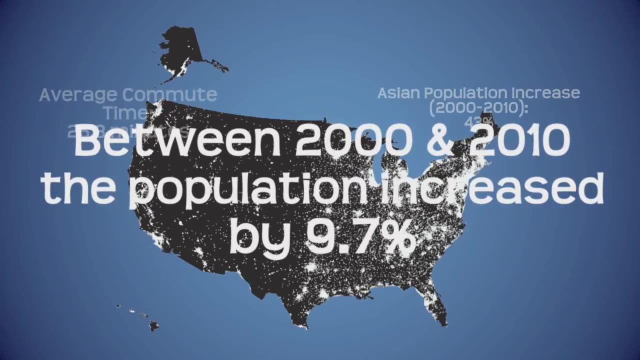 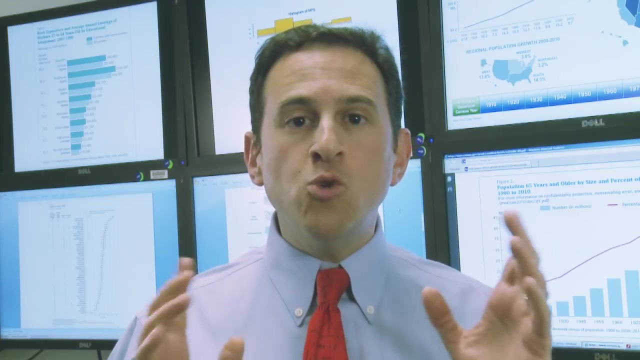 too small. Now let's consider the kinds of questions that we answer with statistics. We talk about things like the population of the United States. The population of the United States In 2010,. there were 308 million people in the United States. You can't possibly know everyone. You can't talk to you, can't you as a person? 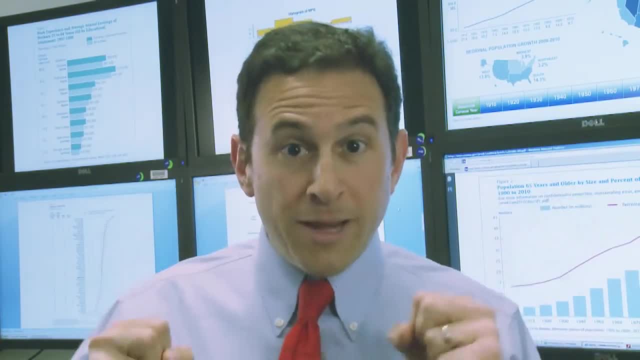 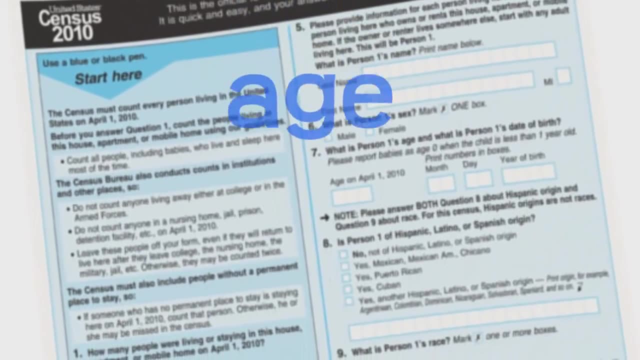 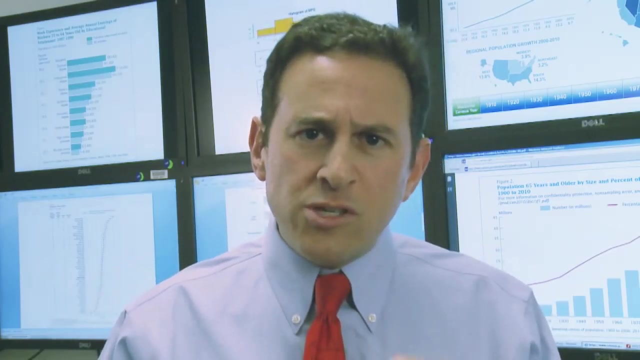 you don't have enough time in your life to sit down with everybody and learn their story, But you know, every 10 years or so we at the Census Bureau ask a few questions of everybody: Age, sex, birth, where you live. These are important things to know, And with just those. 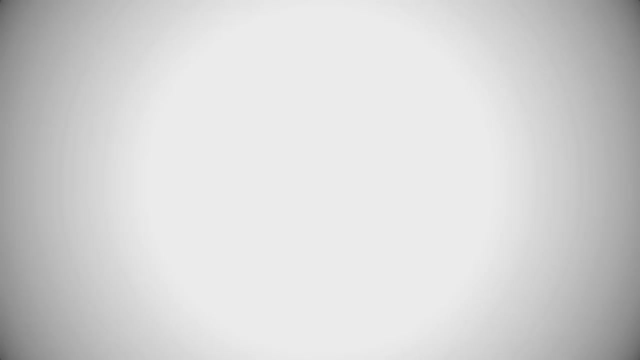 few questions we can learn an enormous amount. You want to know where the hospitals go. You need to know what cities have a large aging population. You want to know where the schools go. You need to know where the cities and what neighborhoods have a lot of really young. 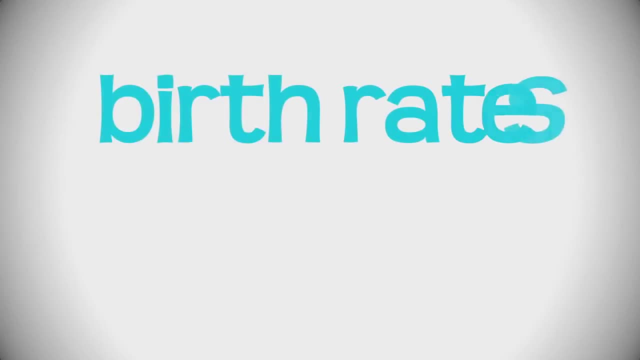 people, These kinds of questions, And it's all kinds of things. You know birth rates, death rates. You want to understand the labor force. That's a statistical question. You want to understand employment. You want to understand earnings. You want to understand. 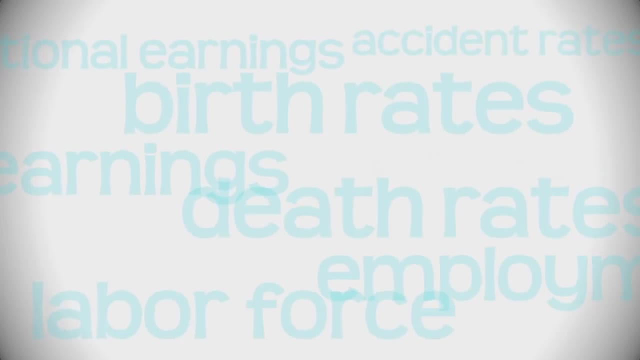 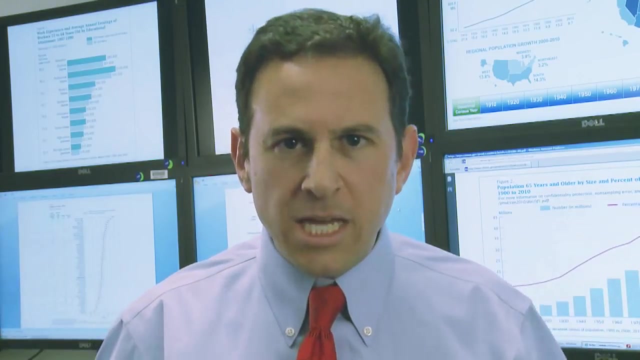 national earnings? You want to understand these questions. Accidents rates, All kinds of things that we publish statistics, on that we measure statistics. They're all things that are too big to see at one time. They're too big for your eye to see. 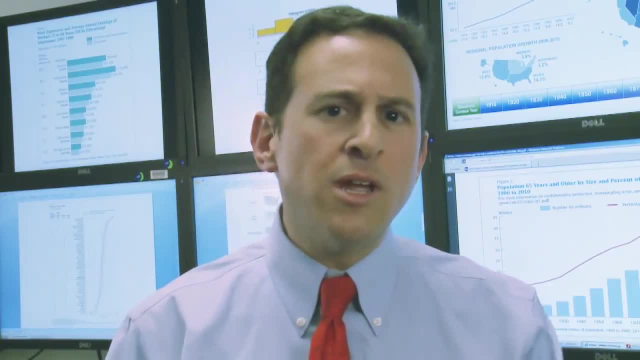 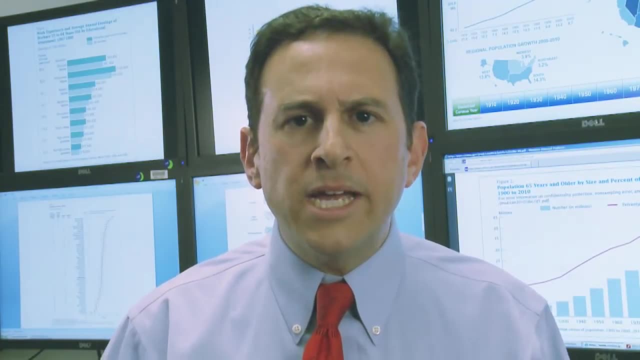 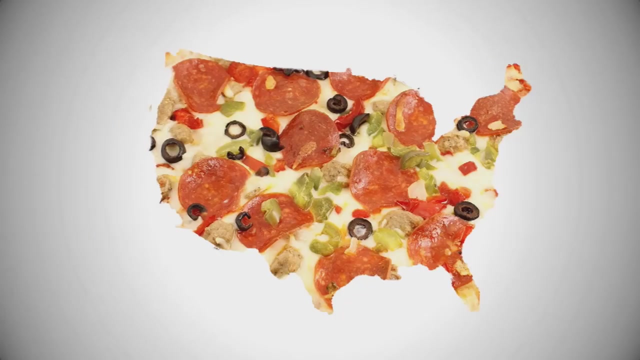 Three hundred and eight million people, all of different ages, all different sex. We've got accidents happening spread out across a country of literally millions of square miles. We can take a slice of that country. We can take a slice of the United States of America.